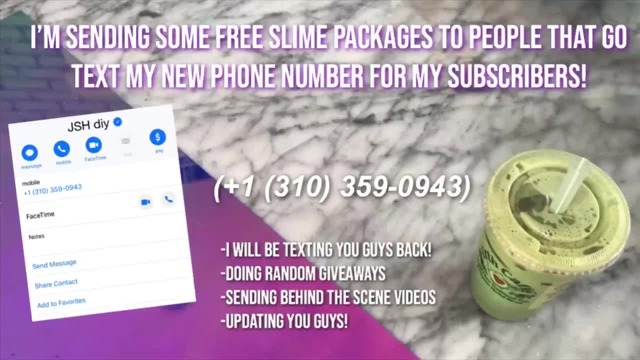 slime recipes. So if you guys have any questions, feel free to leave them in the comments below. I do giveaways and I also just respond back to you. It's actually me, so go send me a text and I will be sending slime packages to people all day long that text me. So go text me right now. 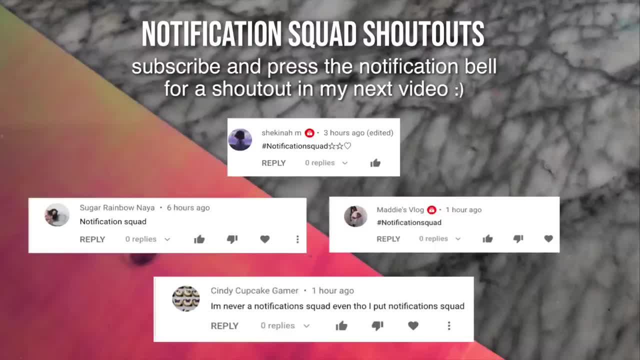 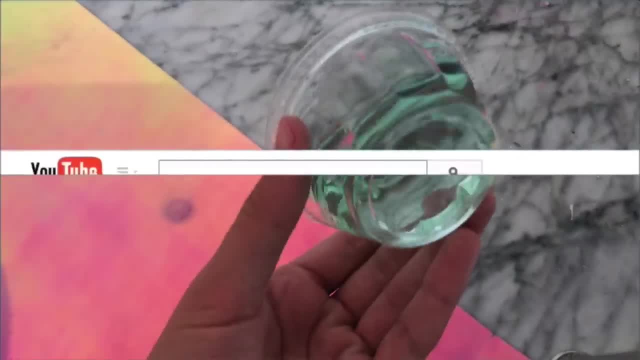 and I will try to send you a slime package. Today's notification squad shoutouts go to Shakirna M, Sugar, Rainbow Naya, Maddie's Vlogs and also Cindy Cupcake Gamer. The first one ingredient- no glue slime we're going to be testing today is mouthwash slime. 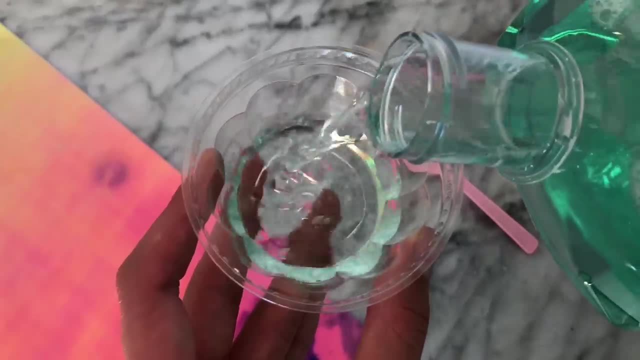 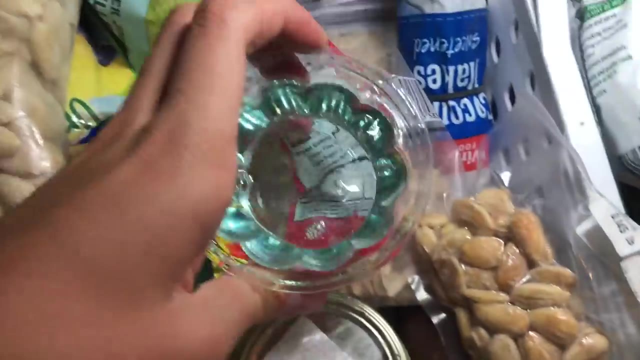 All you're supposed to do is freeze alcohol-free mouthwash in the freezer, and you are allowed to add one pump of hand soap if you want to make your slime extra thick. It has been two and a half hours now since I actually put the Listerine in the freezer, so I'm very excited to see what has. 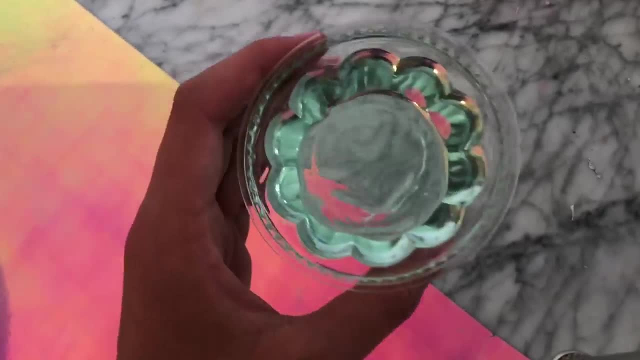 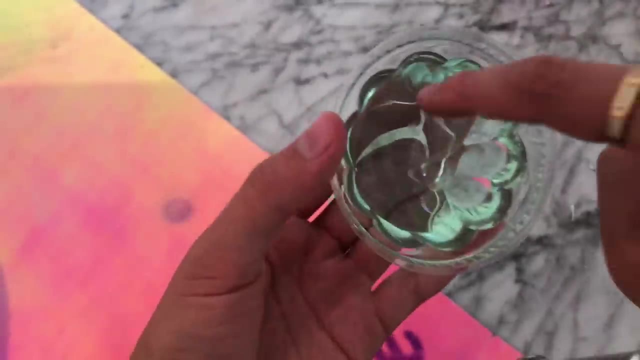 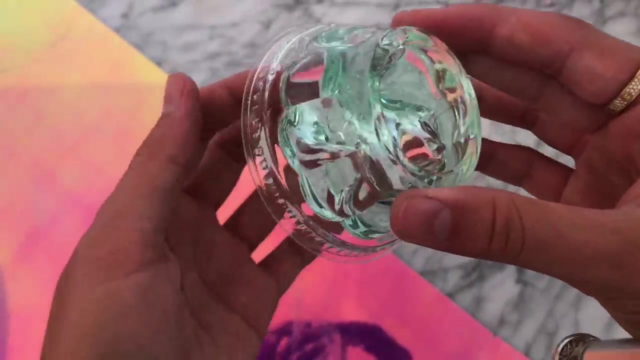 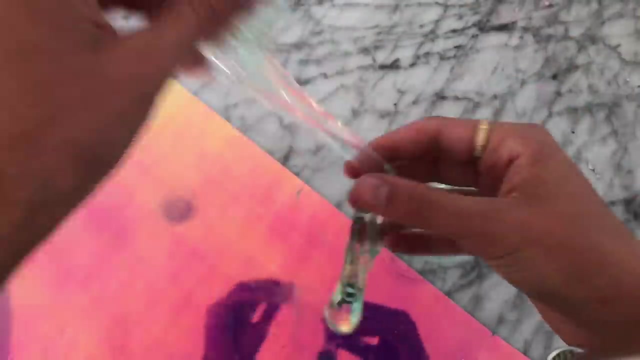 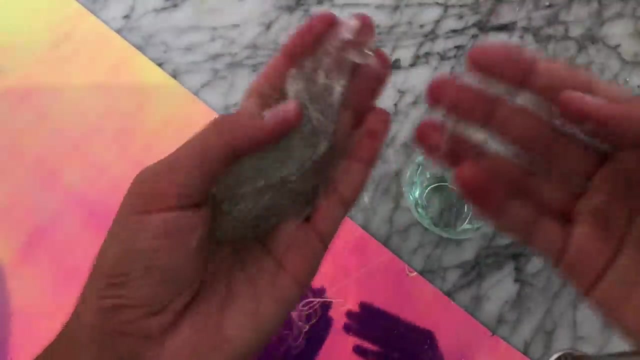 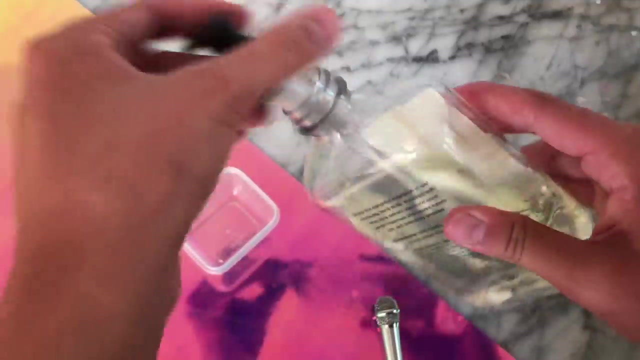 happened to the Listerine. The Listerine had some sort of a reaction with the hand soap, except for I wouldn't say that this was a successful recipe, because it's not something you can hold and play with. For this next recipe, I'm going to be showing you guys how to make a one ingredient hand soap. 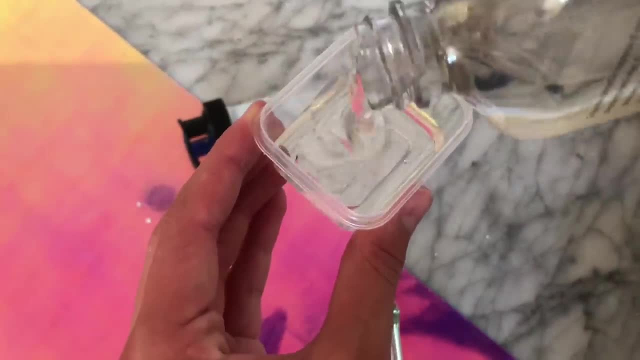 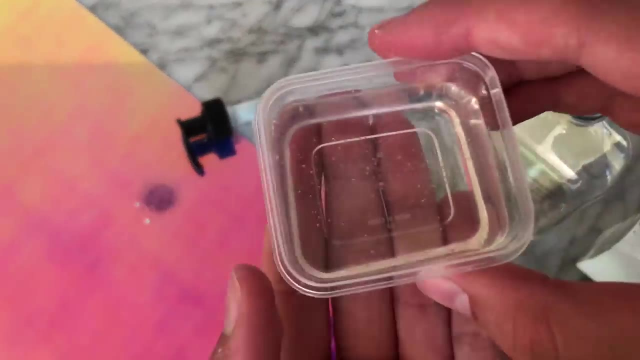 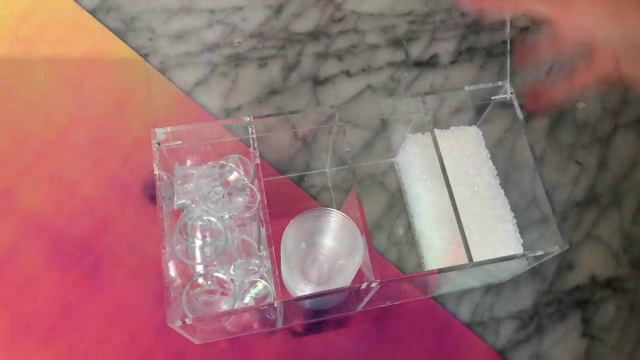 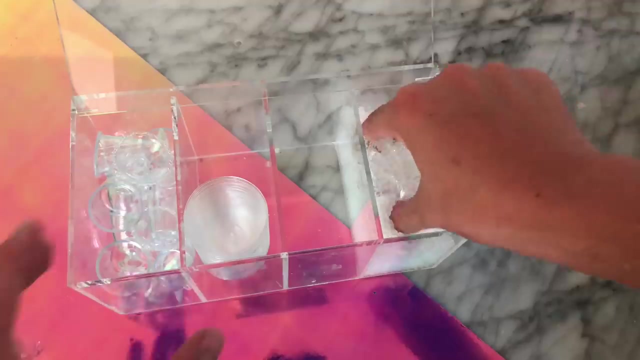 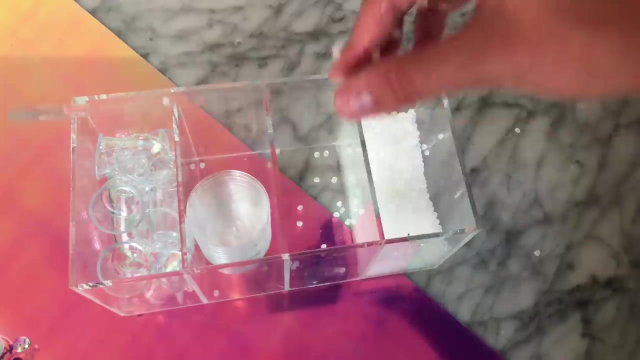 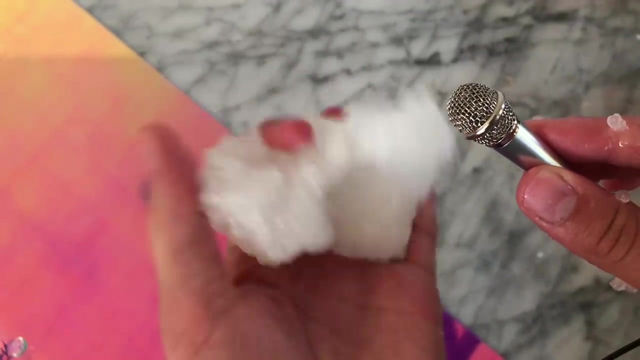 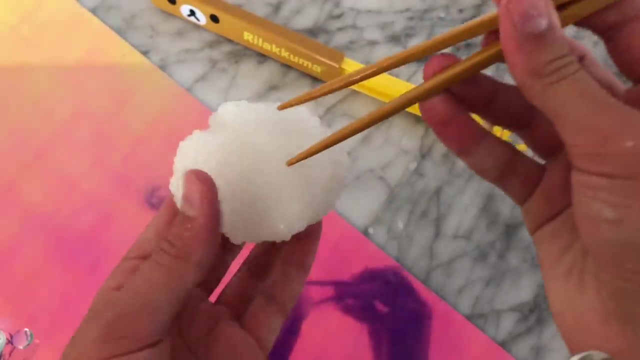 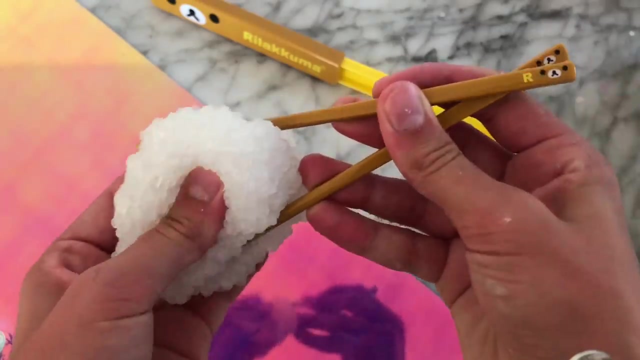 clear slime For activation. all you need is the smallest little sprinkle of salt, Leave it overnight for it to dry and you'll get this. I'm going to add a little bit of beads into this slime to make it a rice slime. This recipe works great as a really playable base slime, and you can really customize this. 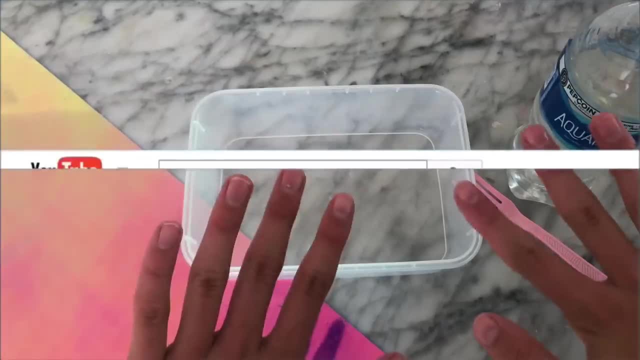 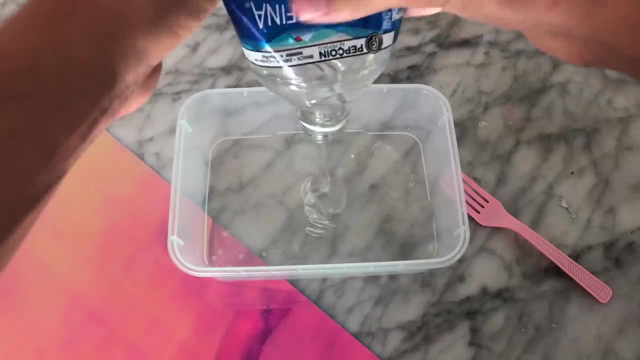 into whatever type of slime you want. I always get requests to show you guys how to fix a sticky no glue slime, so today I'm going to be showing you guys how to. The slime I'm going to be fixing is a sticky no glue slime. I'm going to be using a sticky no glue slime. 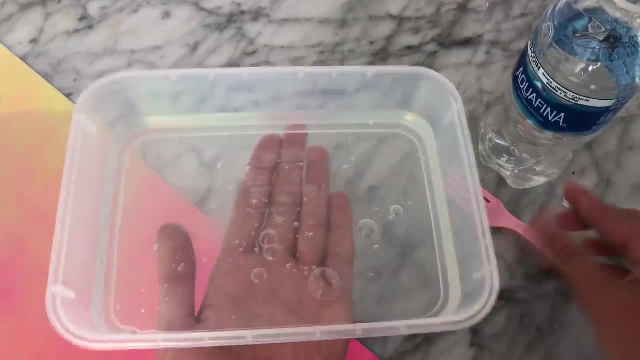 I'm going to be using a sticky no glue slime. I'm going to be using a sticky no glue slime. The slime I'm fixing today is a shampoo slime that did not work for me, As you guys can see. this is not holdable. 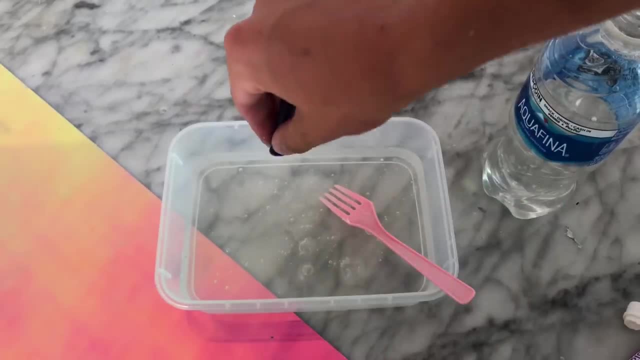 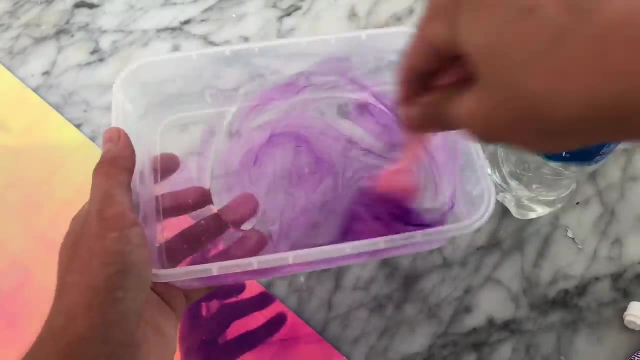 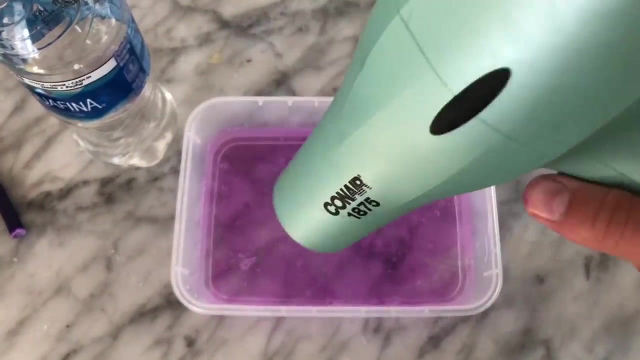 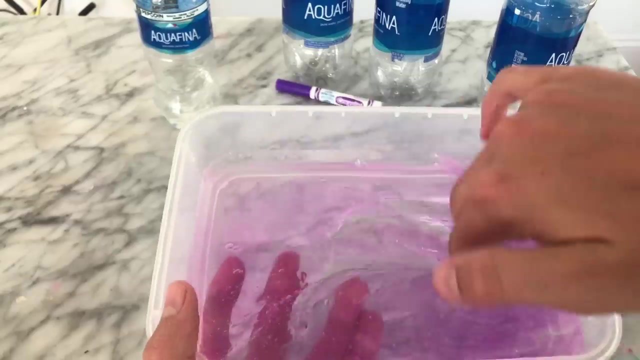 First I'm going to add some marker to color the slime, To make the slime not sticky anymore. you will need a hair dryer. You'll know you're done drying when you can touch the surface of the soap without sticking. You guys can see it's still a little bit sticky, so I'm going to put a container lid on it and we'll let this sit overnight. 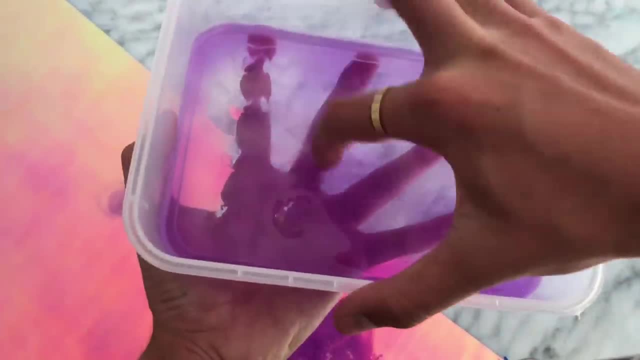 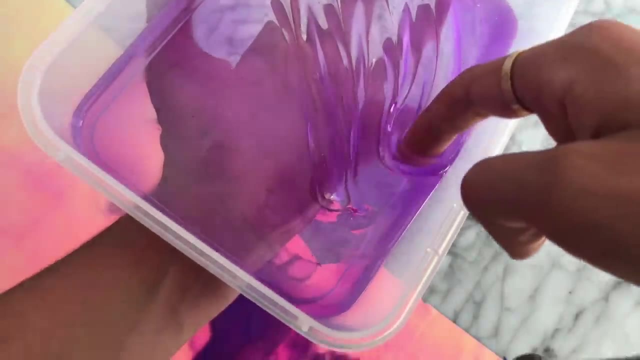 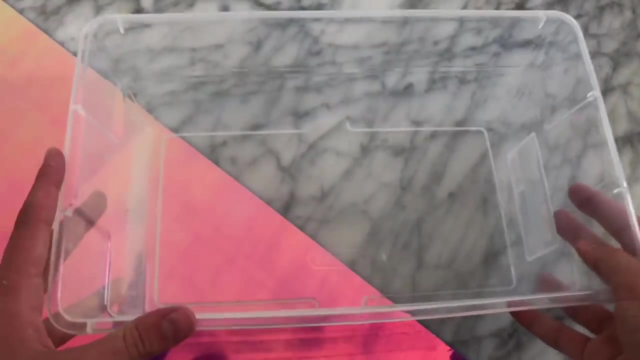 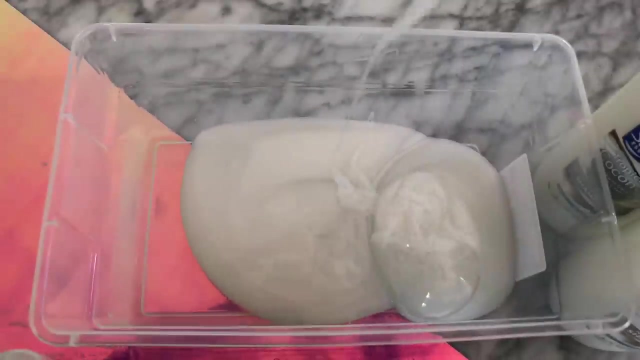 Here's the final result. As you guys can see, you can now poke the soap slime without it sticking to your fingers at all. Since the beginning of the week, you guys have been asking me to try putting shampoo in my hands, but guess what? I have now let this dry out for a couple hours. 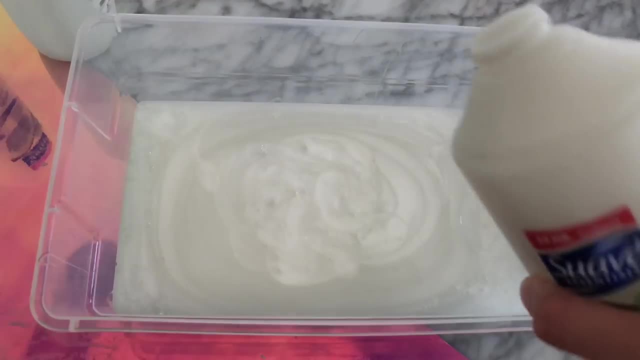 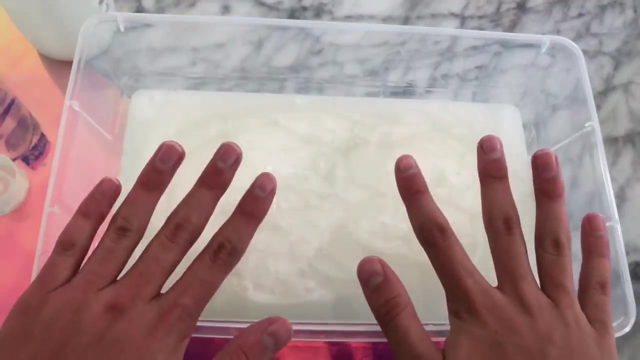 to see if it will turn into slime. I'll be adding this pack of soap slime- and that's the honest view on my body- before I startトüаying the slime- Same technique as the other time: my whole body started to ripen. Okay, so I have my container on. now I'll be adding dry cleaning ethanol. This is this good looking top care for my skin. I usually normally put some in the ask question right, sometimes looking for good quality‌…. here I am. I don't really really know why. what I am doing every day tät to misuse it a bit. This is what I'm actually going to do. This is what I did with this top care. So my two 6 months in camera. I'm going to mix it with a little fish stock and let this sit overnight and I'll leave it quiet for 10 minutes in the afternoon. 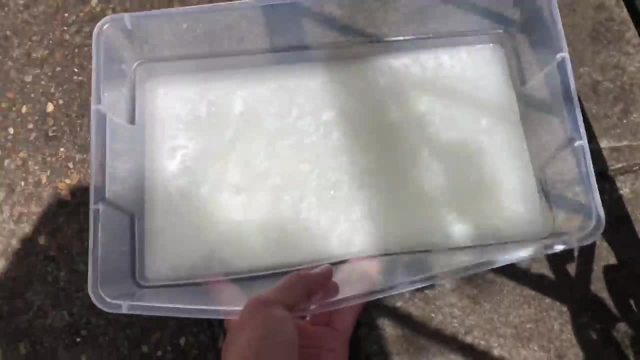 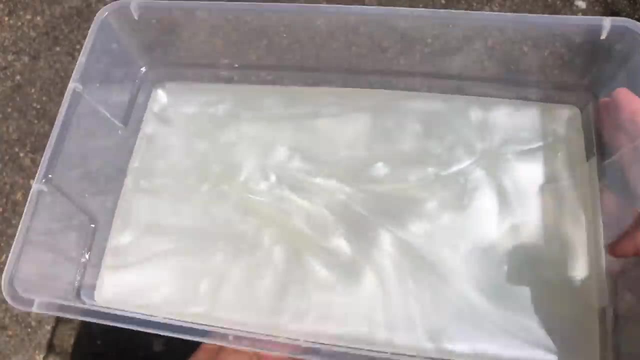 or until i give up. okay, guys, it has only actually been probably 30 minutes. i was expecting it to take a couple hours, but i left it out there for 30 minutes and i feel like it might have actually dried out a bit. so i don't know if this is picking up on camera, but you guys can see the top layer of 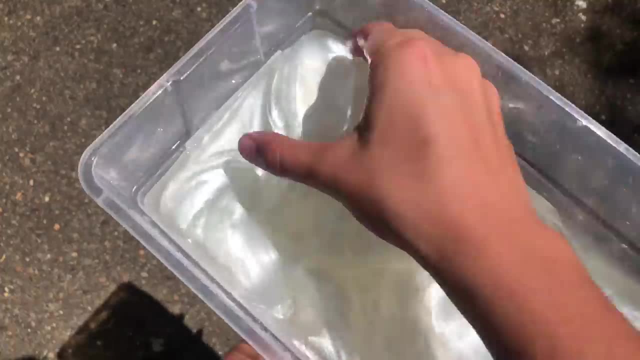 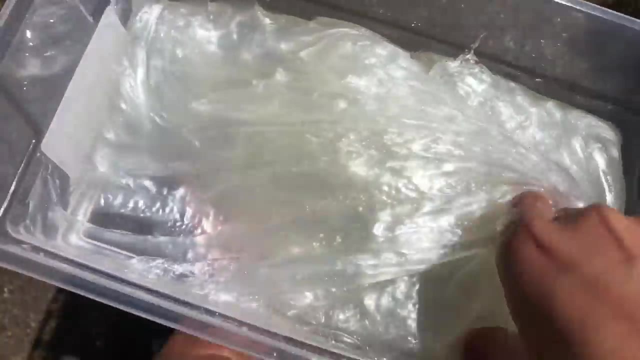 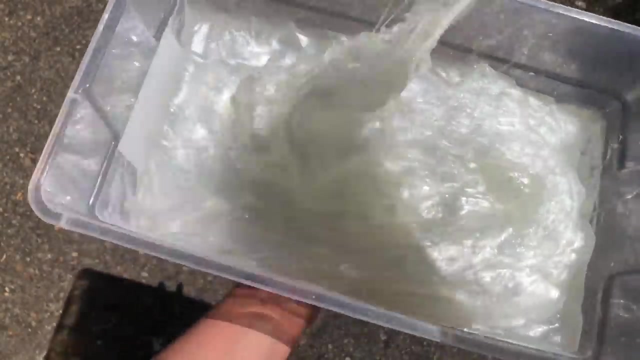 the shampoo feels kind of dry, but at the very bottom of the batch it feels like a really liquidy version of the shampoo and it almost feels like it has melted. so this has a really inconsistent texture. it is 100 thicker than before but it feels runnier in some spots, so it's a little bit. 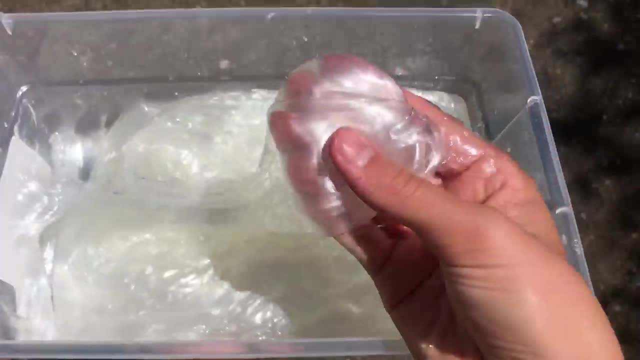 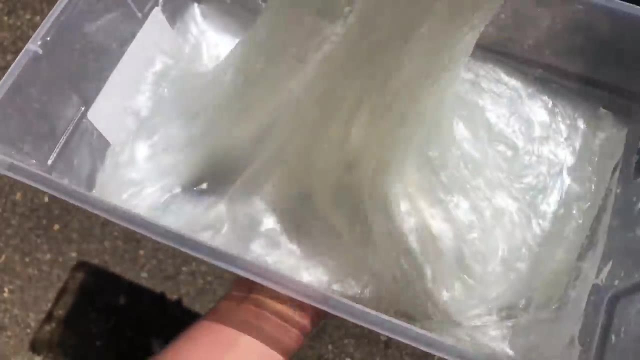 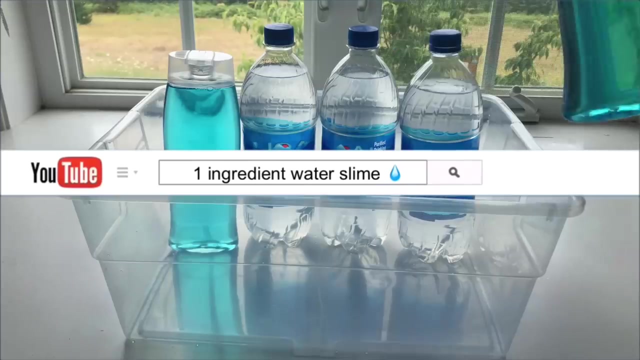 weird, but this recipe did work- like i could totally see this working for some people because it pretty much worked for me. but let me know in the comments if you guys have tips to make this make more of a consistent, better slime texture. for the past month or so i've been trying to find the perfect one ingredient: water. 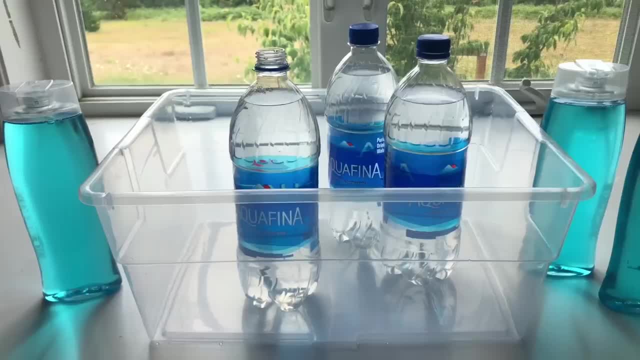 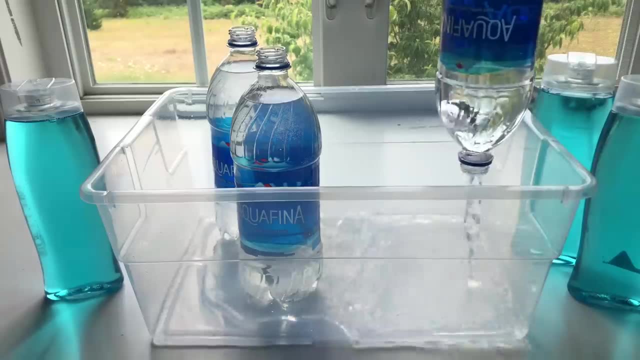 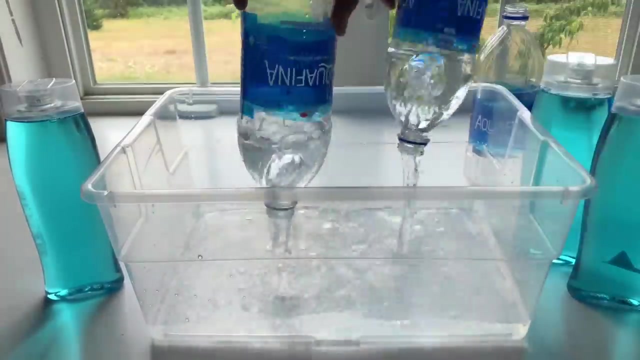 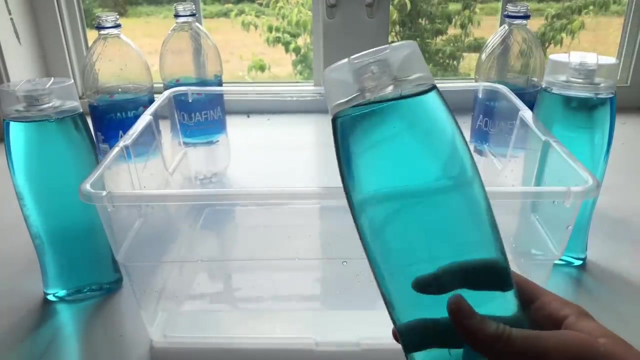 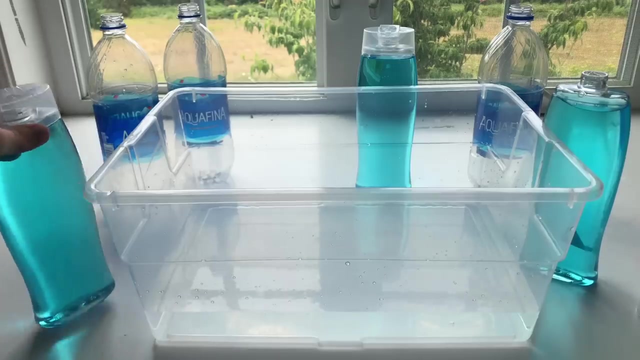 slime. so today i'm going to be showing you guys how to make one ingredient: water gel. for the recipe, all you need is any shampoo and, of course, water. life is what it is right now. right now, tell me now, cause i don't know what i'm supposed to do. i just wanna be right next. 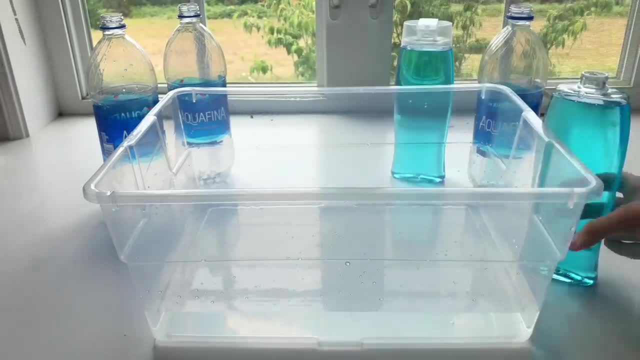 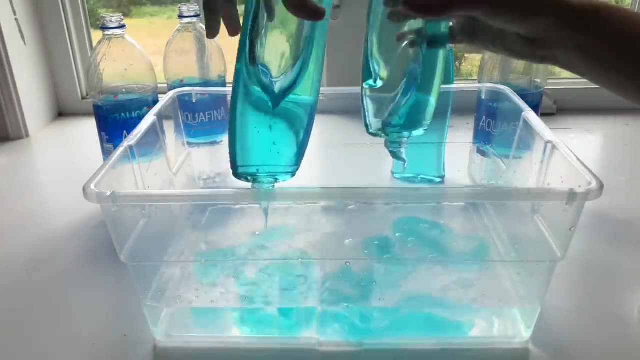 to you, even though i try to get you off my mind. you know that i'm thinking about you all the time, like when we were driving in her car, looking at the stars made us stop at every bar we found. i can see. it's like a movie in my head. 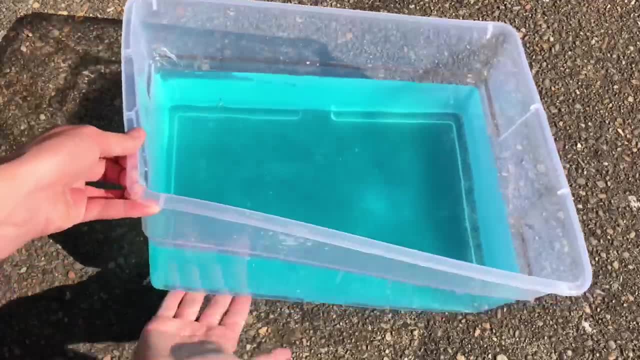 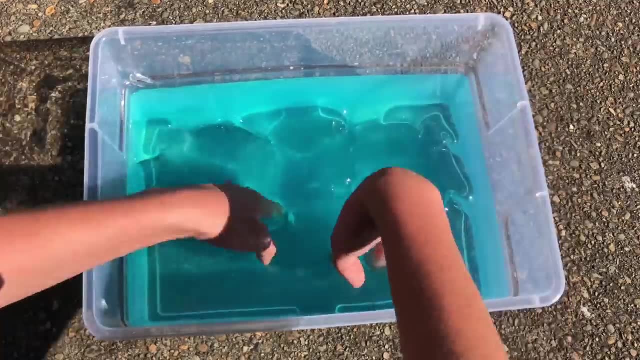 here is my finished slime. i had to let mine sit to dry out and clear up for, i would say, around a week, which took a while, but it was definitely worth it because, as you guys can see, it gives you a really nice. it gives you a really nice gel. 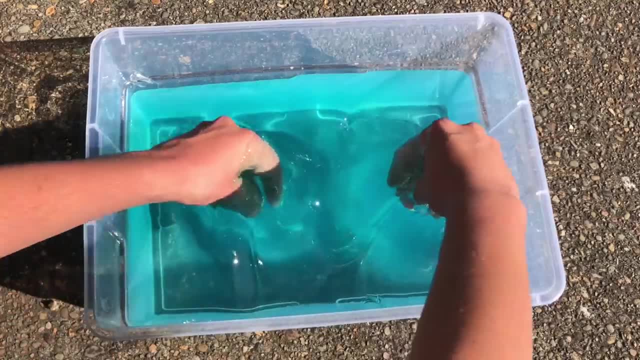 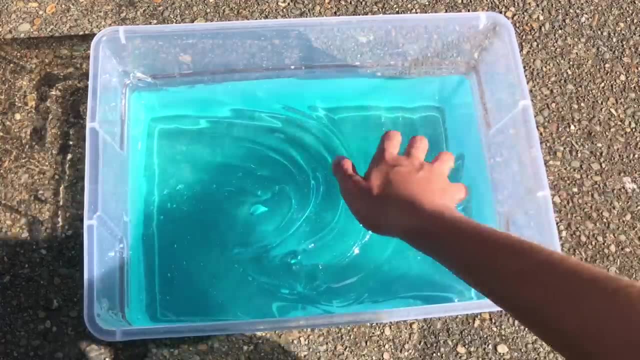 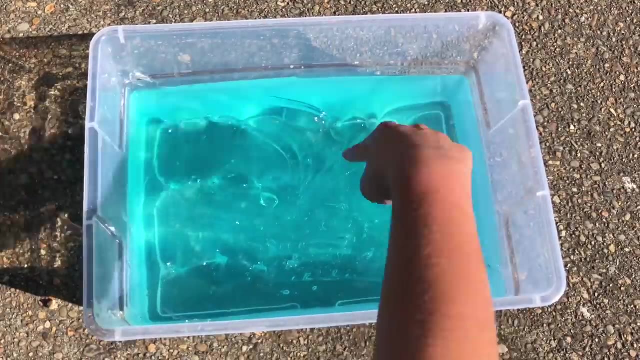 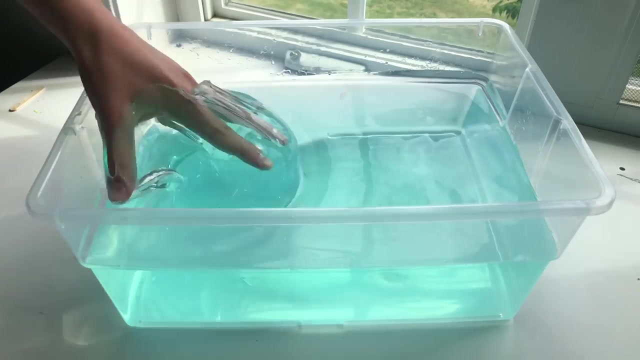 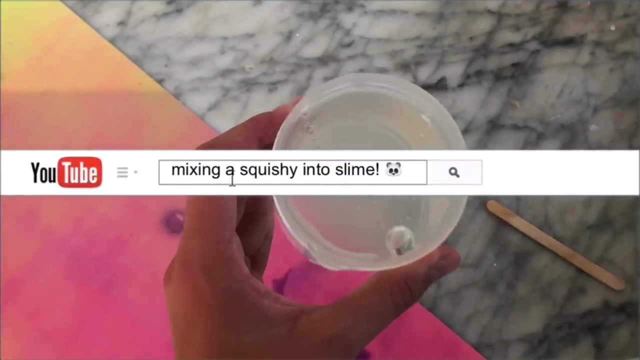 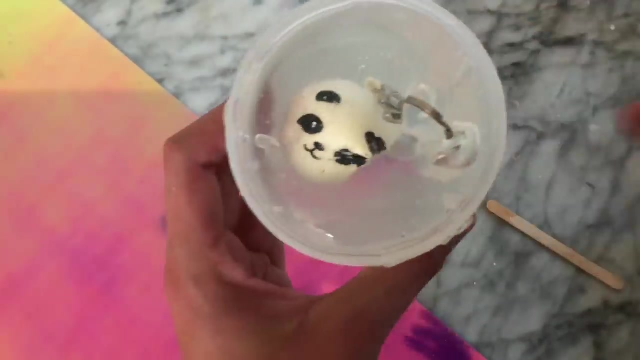 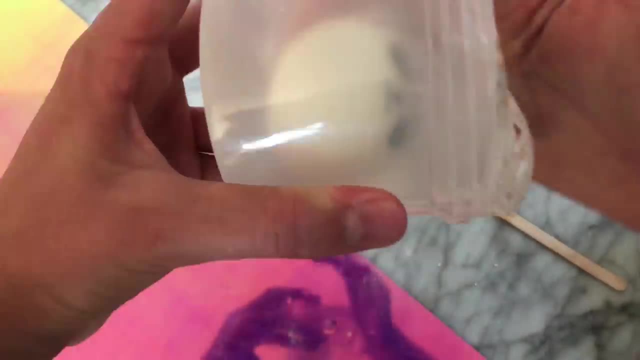 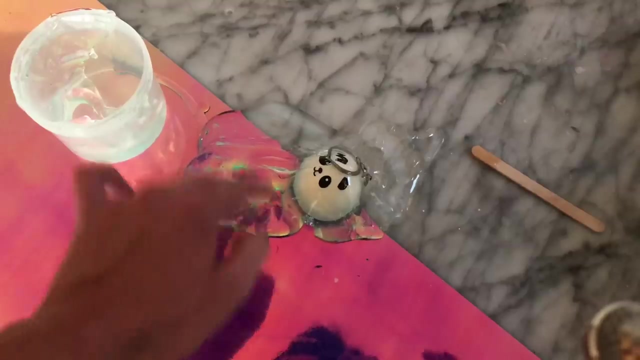 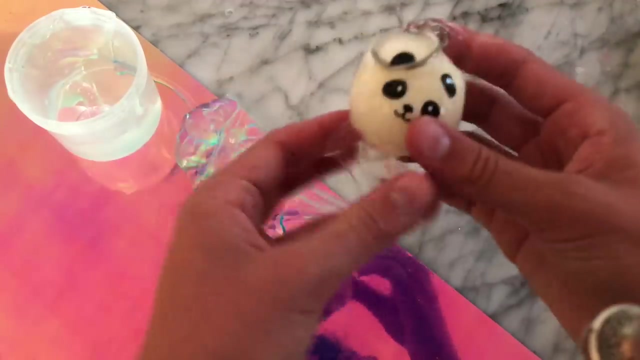 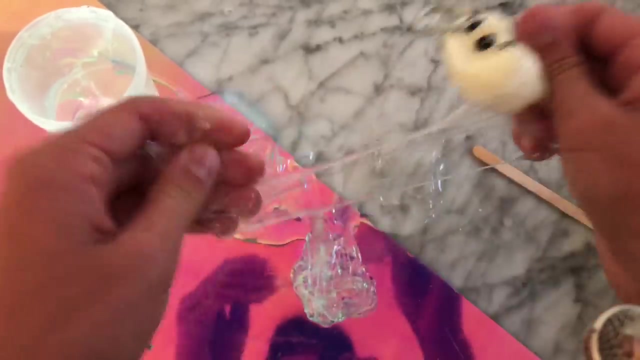 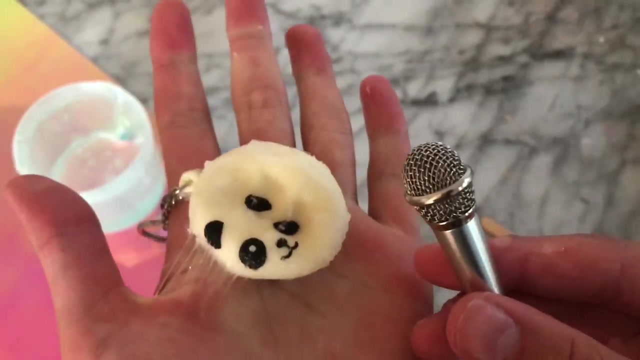 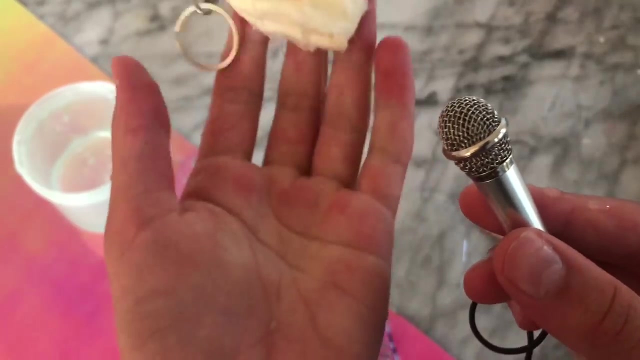 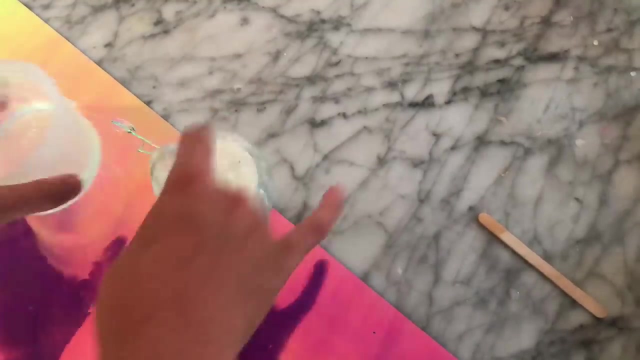